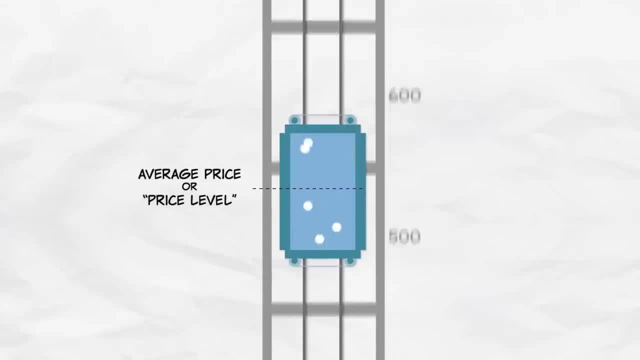 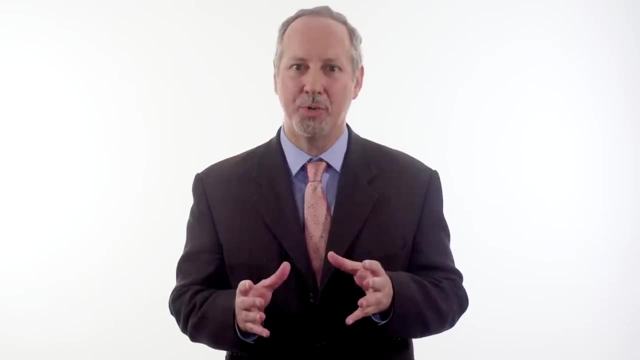 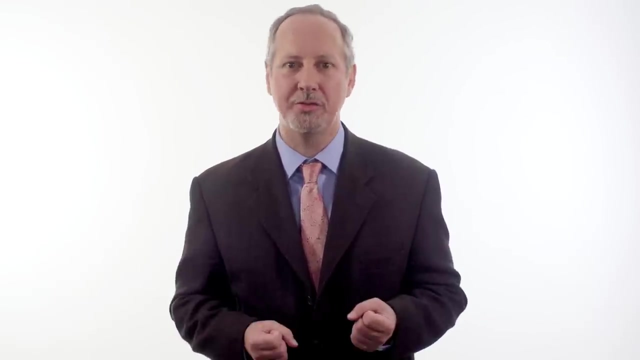 Now. inflation is when the average price is going up. Inflation is when the elevator is going up. We measure the average level of prices using a price index: the average price from a large and representative basket of goods and services. There are different price indexes that are based upon different baskets. 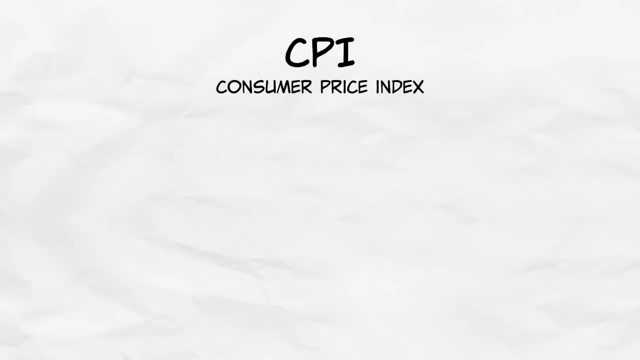 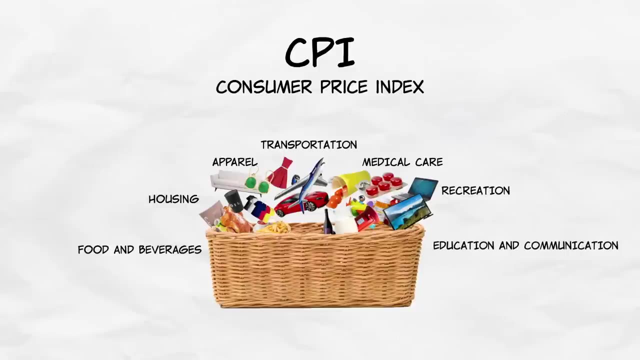 The Consumer Price Index, or CPI. it's based on a basket of thousands of goods and services which are bought by consumers in the United States And it's a weighted average, so that an increase in the price of a major item like housing that counts for more than an increase in the price of a minor item like toothbrushes. 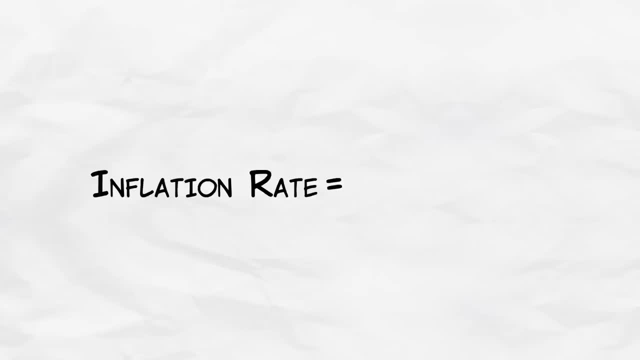 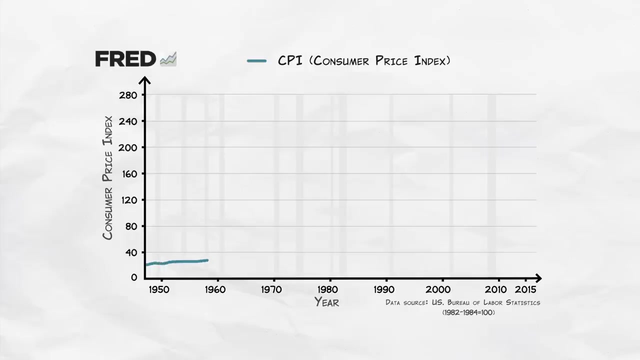 The inflation rate can then be measured as the percentage change in the index over a period of time, say a year. So let's take a look at the inflation rate in the United States as measured by the CPI. If we Google inflation United States, FRED, we'll find a graph like this: 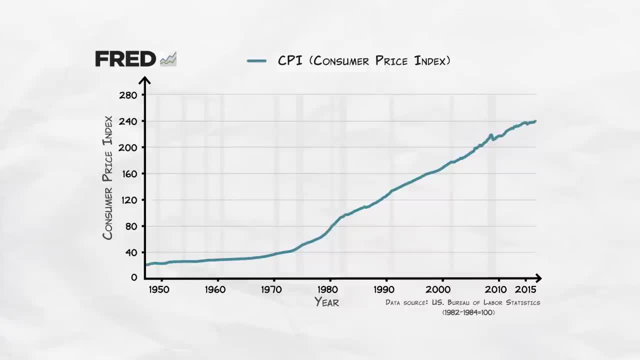 The graph shows us the CPI. Now, this is a graph that shows us the CPI. Now, this is a graph that shows us the CPI. Now this is a graph that shows us the CPI. The index is defined so that the average price in the years 1982 to 1984, that's set equal to 100.. 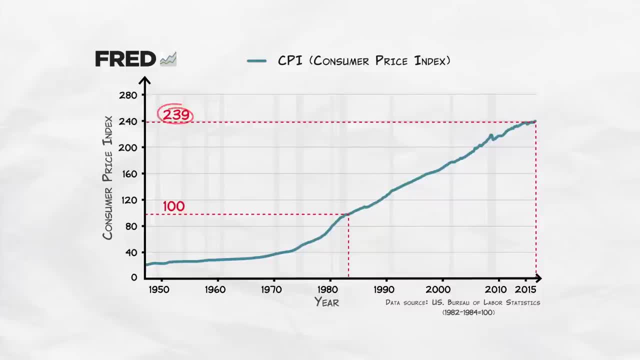 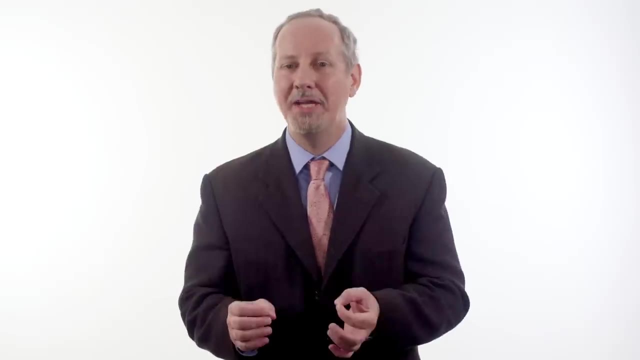 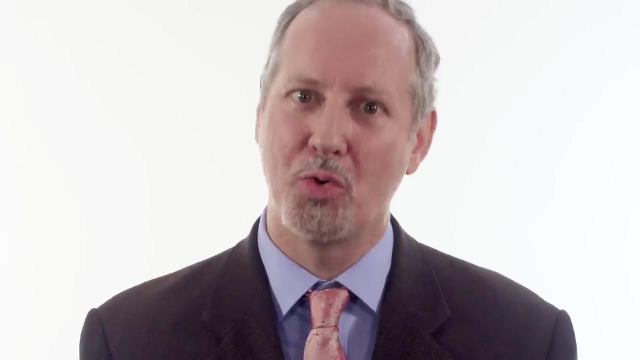 In mid-2016, the index was 239.. So that means that over the past 33 years, prices on average have more than doubled. Now that doesn't mean that we're necessarily worse off today than in the past, Because wages also gone up over this time period and in fact, wages have gone up on average by more than prices. 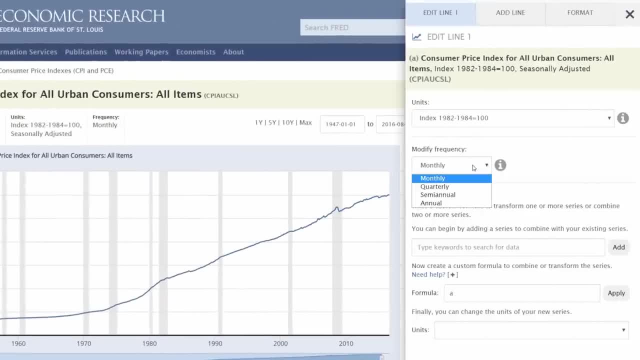 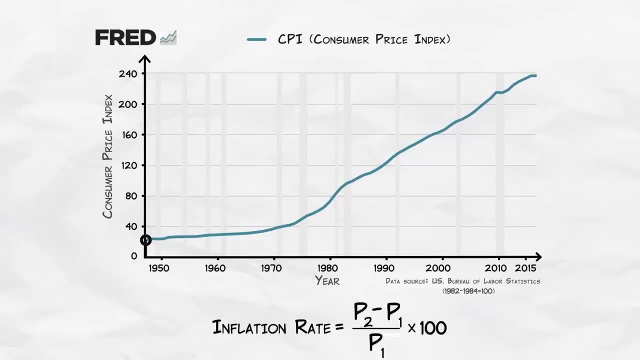 by clicking on edit data series we can change to an annual series. now we can see that in 1973 the cpi was 44.425 and in 1974- the average price of the cpi basket it had risen to 49.317. we can now calculate that the rate of inflation over this year was 11.01.